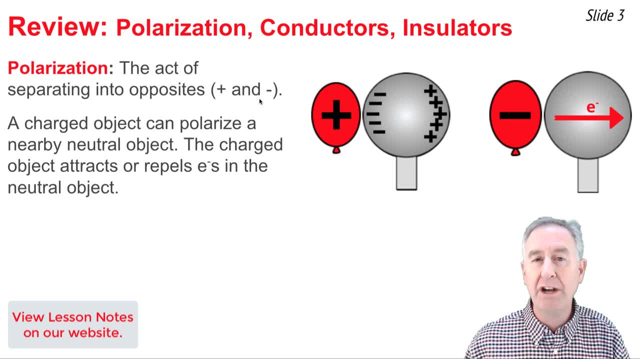 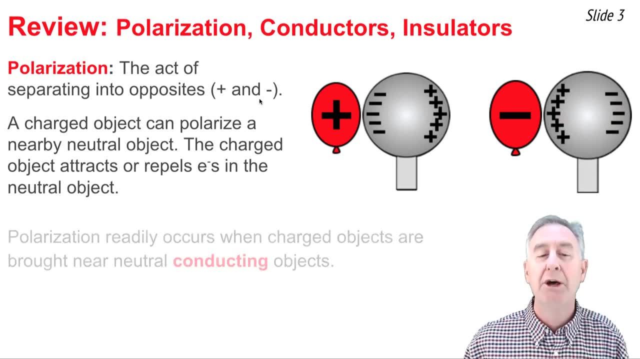 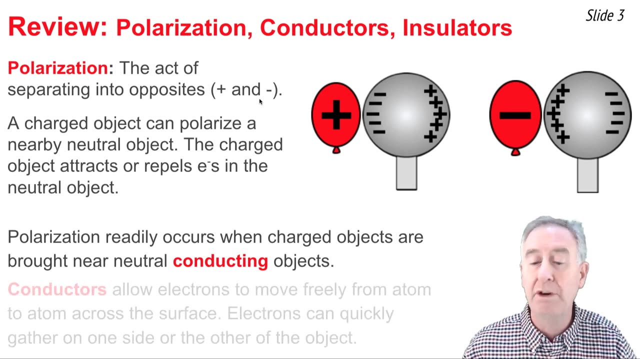 direction, as they are repelled by the negative balloon, So electrons move within the neutral conducting sphere. Polarization occurs much more readily in conductors than it does in insulators, and that's because conductors allow for the free flow of electrons across their surface. 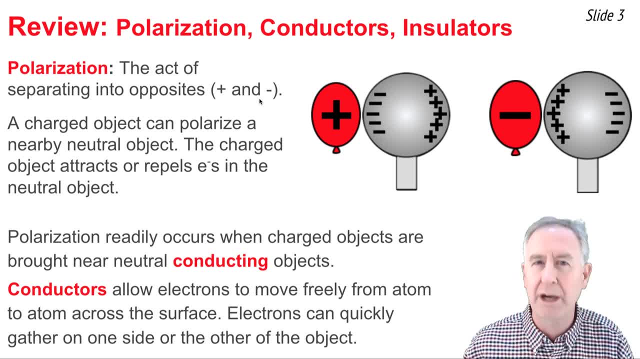 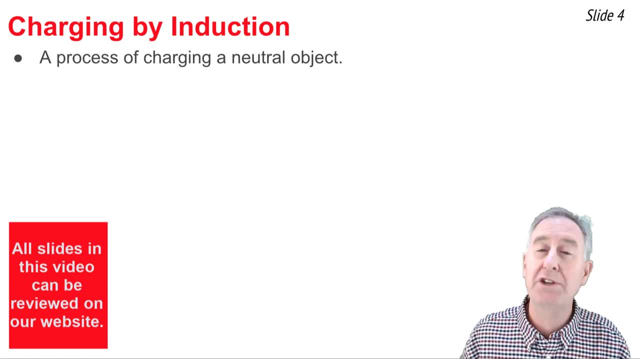 and so they can gather up on one side or the other when induced to move by the presence of a nearby charged object. Charging by induction is one of several charging methods that are used to charge a neutral object. The procedure goes something like this: First you start. 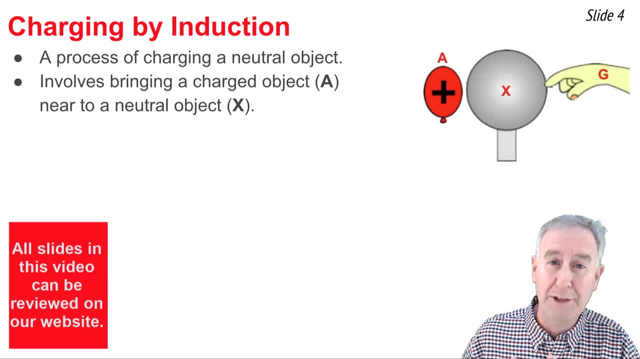 with an object which we'll call object A. It's the positively charged balloon that you see. It's brought near a neutral object, which happens to be the gray sphere sitting up on an insulating stand. We'll call that object X, While object A is held near object. 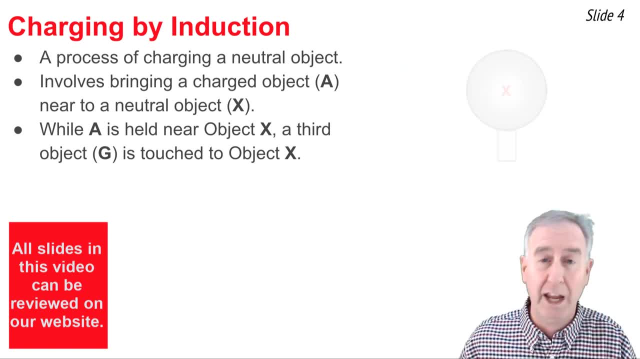 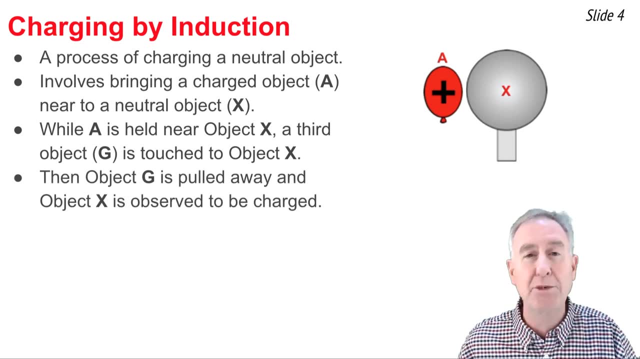 X. a third object is brought nearby. It's the finger or hand that you see. We'll call it object G, where it stands for the ground. Then it is touched to object X and finally object G is pulled away, and at that point you would observe that object X has become. 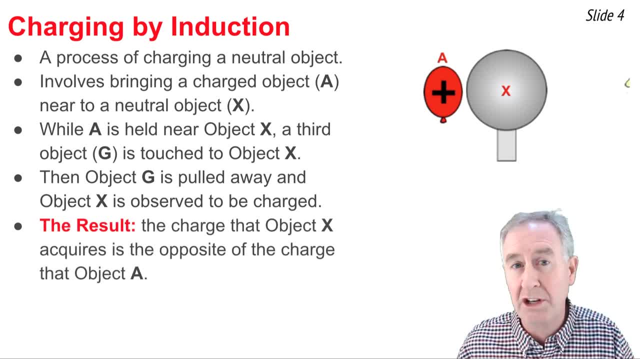 charged, And the result of this charging process is that the charge on object X would be the opposite of the charge that object A has. So in this case object X would become charged negatively. Two important things to note here. First, there's never any contact. 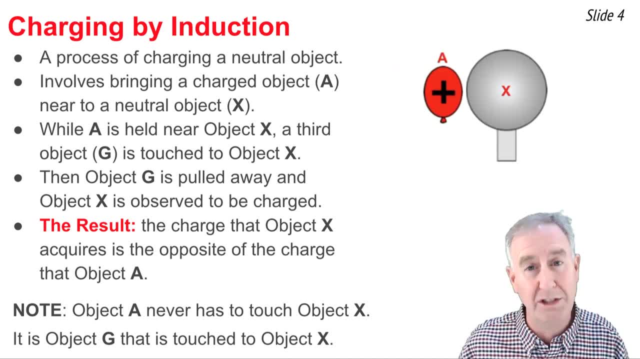 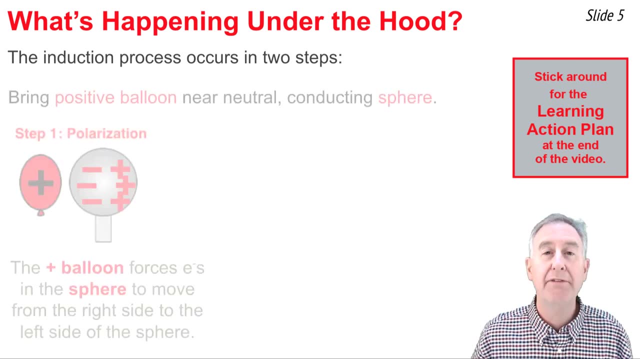 made between object A, the balloon, and object X, the sphere. Second, the only contact that ever is made here is between object G, the hand, and object X, the sphere. To understand by induction process you have to think in terms of two steps. In the first step, the 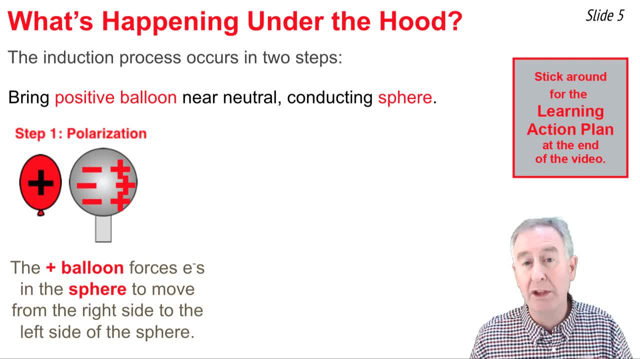 polarization step. a charged object is brought near the neutral conducting sphere. That positively charged balloon is there to polarize the neutral conducting sphere. Electrons within the sphere which are charged negatively are drawn towards that positively charged balloon and migrate across the surface of the balloon to get closer to the positively charged balloon. This is 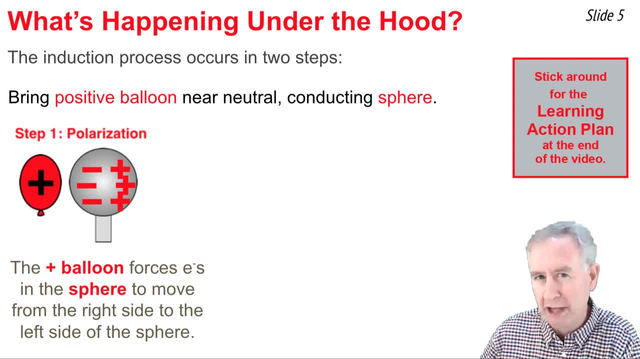 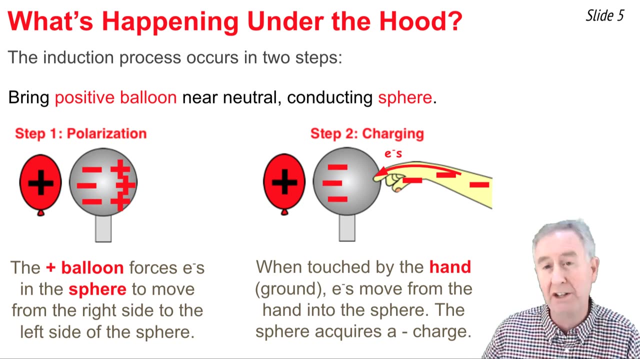 just opposites attract. At the end of the polarization step, the neutral conducting sphere has negative charges lined up on the left side and positive charges on the right side. The second step is the charging step. That's when the hand comes in and touches the right side of that neutral conducting sphere And the result is that electrons within 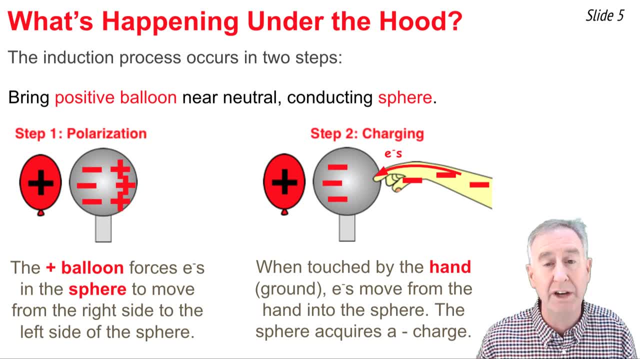 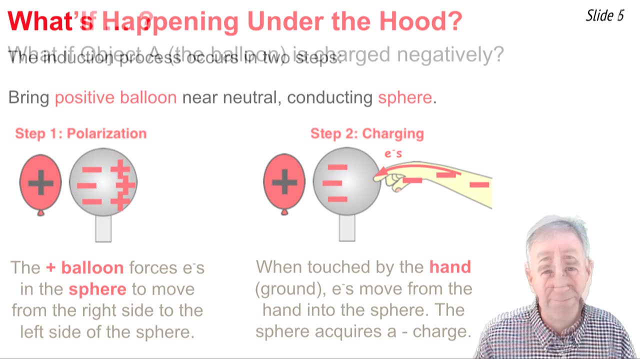 the hand are drawn in to the right side of the sphere, neutralizing the positive excess charge that's there. That also is opposites attract. It's at this point, when the sphere has gained charges, electrons, from the hand, that it acquires a negative charge. 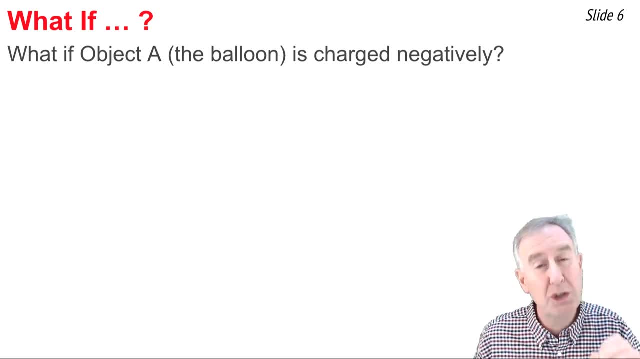 Now what would happen if this balloon that we've been talking about is charged negatively? If object A is charged negatively, then that means that object X is going to acquire a negative charge. How does it happen? We can explain it once more in two steps, with the: 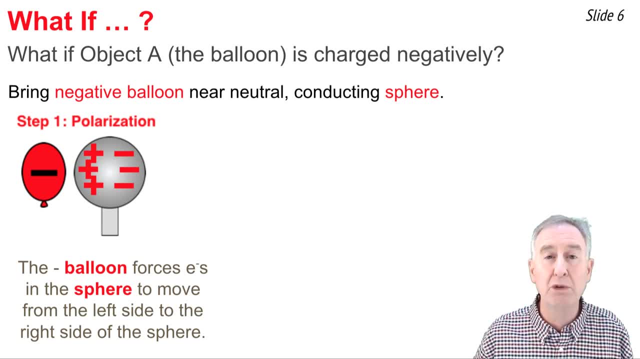 first step being the polarization step. The negatively charged balloon forces electrons within that sphere to be repelled away from it, And they move from the left side of the sphere to the right side of the sphere. That leaves an excess of positive charge on the left. 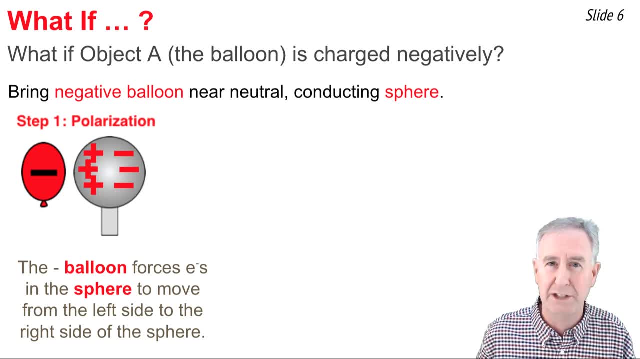 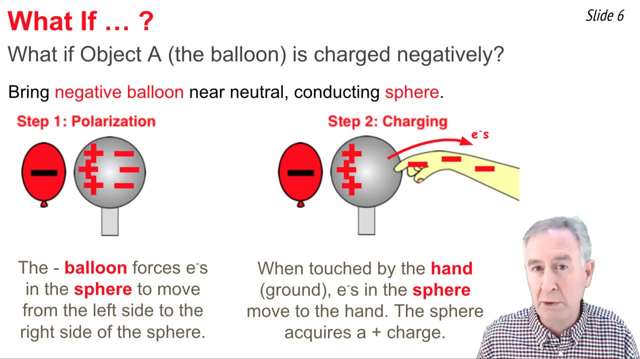 side of the sphere and excess of negative charge on the right side of the sphere. The second step is the charging step, And that's when the hand comes in and touches the sphere, And now, at this point, electrons will leave the sphere and enter into the hand. They're pushed out by the repulsions. 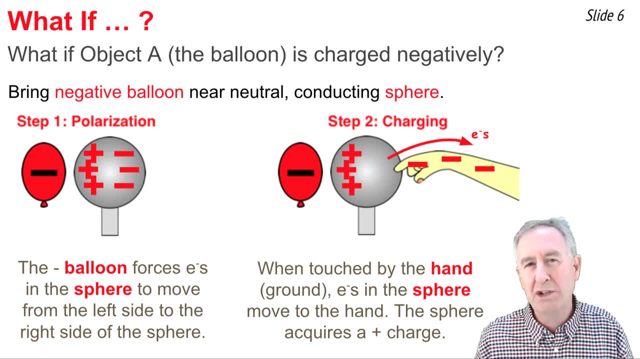 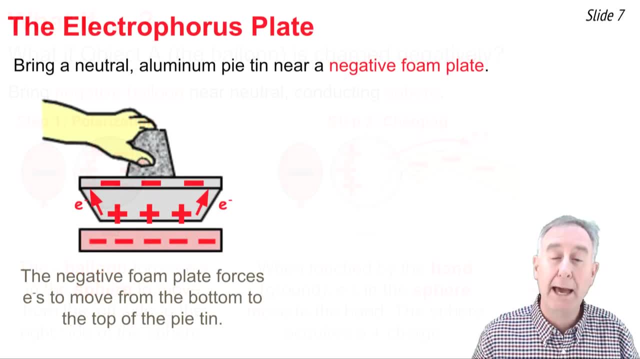 they experience with that negatively charged balloon. This charging step leaves the sphere charged positively since it's lost the negative charge, And that's when the hand comes in and the electrons leave the sphere. A common lab in a physics class is the electrophorous lab, in which you charge an electrophorous. 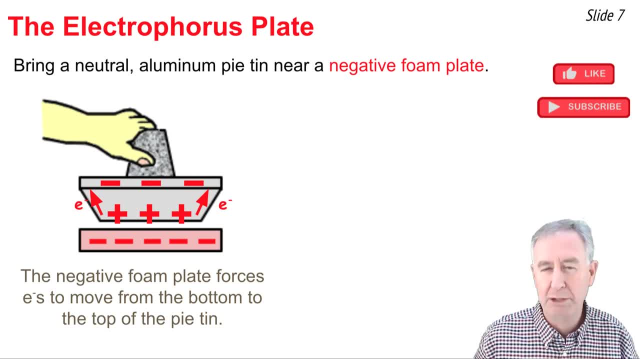 plate by induction. We're just going to call that electrophorous plate an aluminum pi-tin, because that's what's usually used. So we're going to bring a neutral aluminum conducting pi-tin near a negatively charged foam plate. The presence of the negative charge on that. 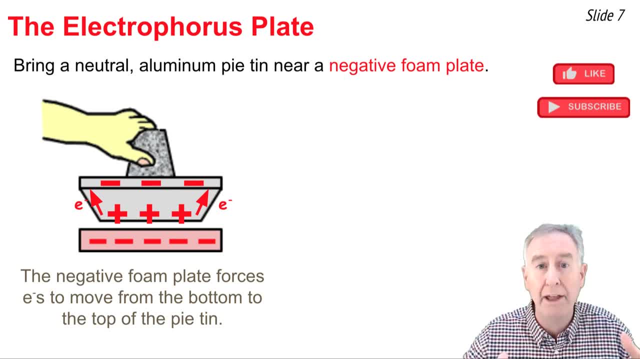 foam plate forces electrons in the pi-tin to be repelled from the bottom of the pi-tin up to the top of the pi-tin, thus polarizing the pi-10.. That's step one, the polarization step. The next step is the charging step. 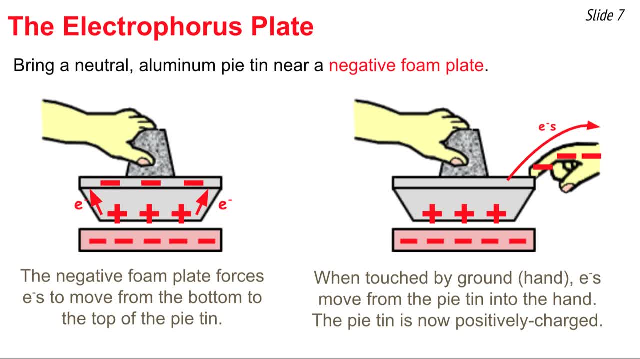 and that's when a ground or hand or finger comes in and touches the pi-10. And when contact is made, electrons leave the pi-10 and travel into the hand. They're still being repelled by the presence of this nearby negative foam plate. 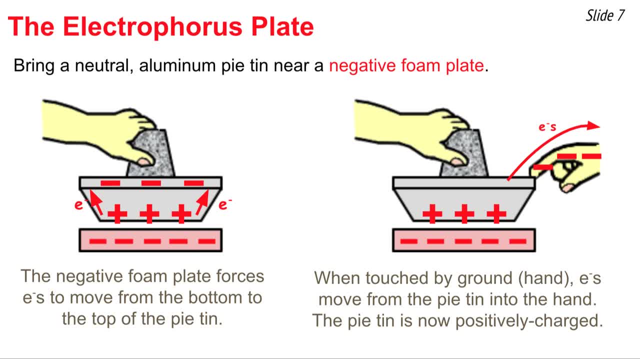 Like charges, like an electron and a negative foam plate will repel one another. So electrons exit the pi-10.. Into the hand, because the aluminum pi-10 has lost electrons, it becomes charged positively. Now we're gonna discuss a slightly different 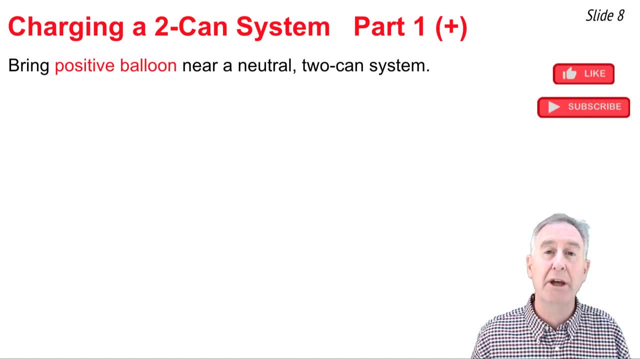 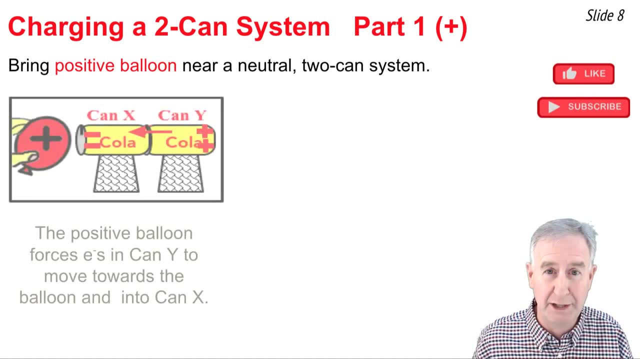 induction charging situation. In this situation, we're gonna bring a positively charged balloon near a system of two neutral conducting pop cans that are touching one another. As we bring that positively charged balloon near the can on the left, which is called can X, 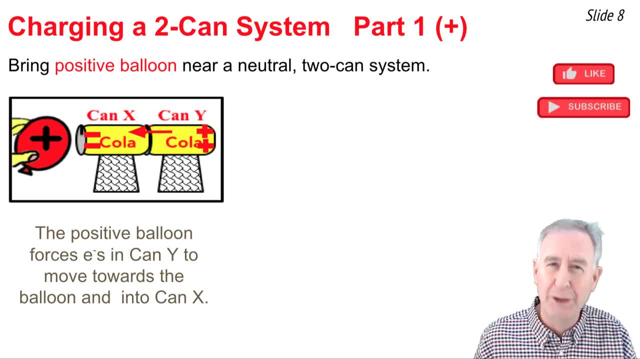 electrons in the can on the right, can Y, are drawn towards the can on the left And that's the positive charge balloon. That's, opposites attract The electrons. leave can Y and enter can X, leaving can X with an overall negative charge. 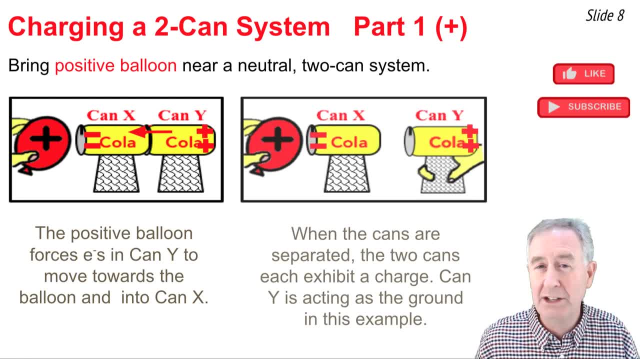 and can Y with an overall positive charge. Then in the next step we simply separate the cans And now X has a permanent negative charge and Y has a permanent positive charge. This would be called induction charging And, using our original model, the balloon is this. object A: 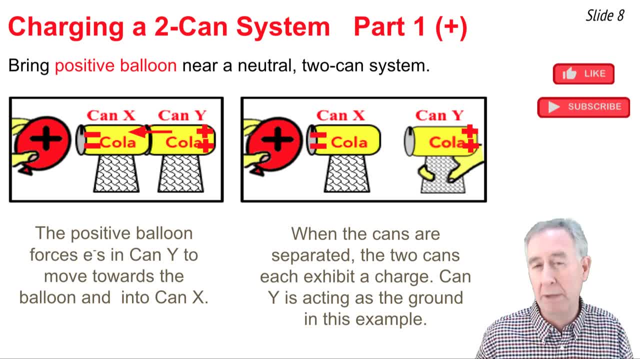 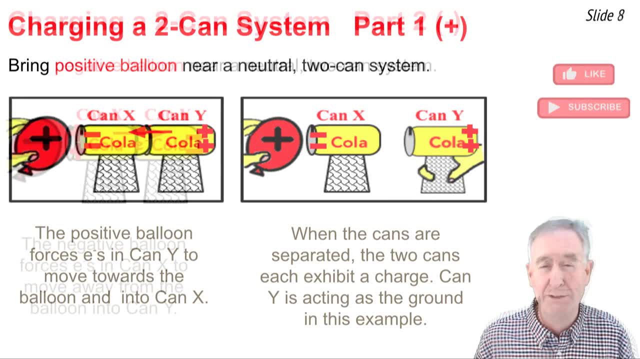 Can X is object A, Can Y is object X, And can Y would be called object G. Let's talk about a very similar situation, but this time with the balloon being negative charged. When the balloon is negatively charged, it works a little differently. 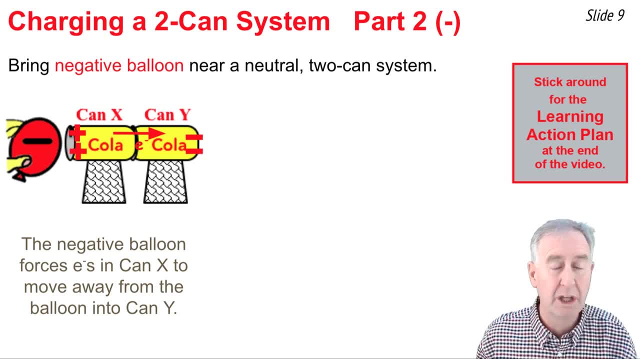 Electrons in can X sense the presence of that negative balloon and they don't like it. So they move out of can X into can Y. That's no magic, That's just the old electrostatic principle that, like charges, repel A negative balloon and negative electrons. 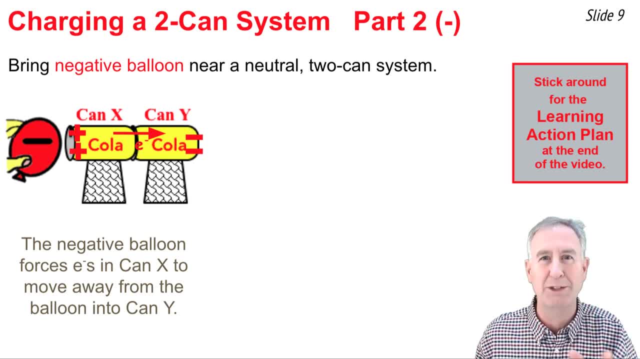 in can X repel one another. That means those electrons scatter into can Y. That leaves can Y with excess negative charge and can X with excess positive charge. Then the cans are separated And when they do, we observe that the can on the left 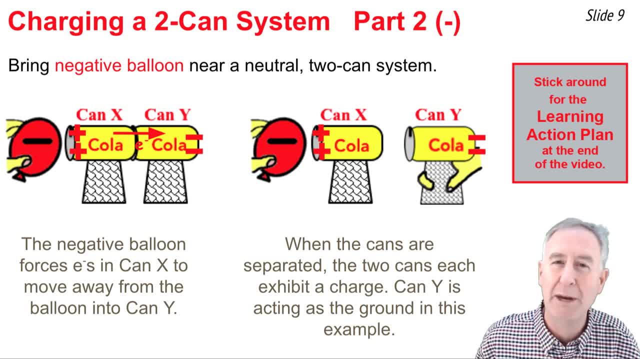 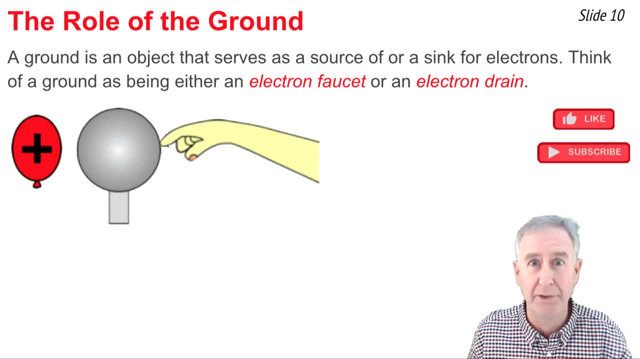 that can X is positively charged and can Y is negatively charged. In our discussions of charging by induction, I've been referring to the hand as the ground. What is a ground? Well, the ground is simply an object that serves as a source or a sink for electrons. 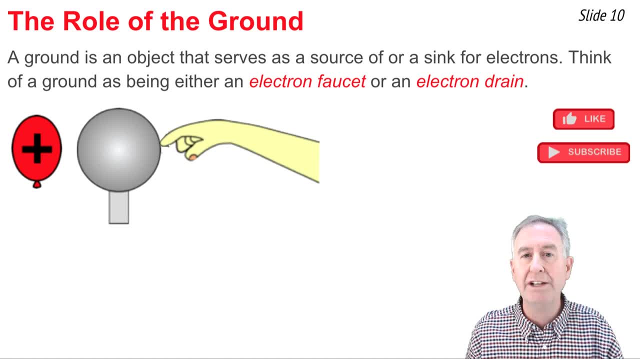 You can think of it as either a faucet or a drain. If electrons are flowing into the neutral object X, then you can think of the ground as being the faucet from which the electrons flow. But if electrons leave object X into the hand, you can think of the ground as being the drain. 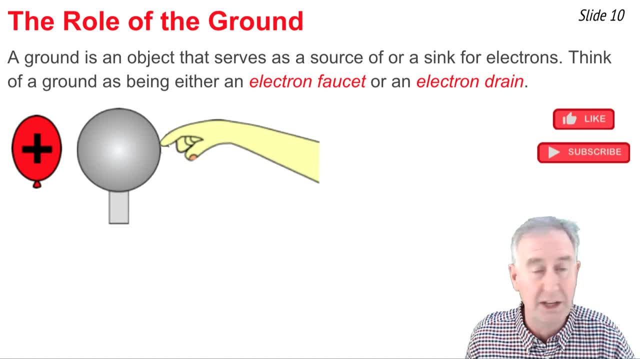 into which electrons flow. So which is it in any given case? And how do you tell? Well, it comes down to old electrostatic principles of opposites attract and likes repel. So what is it? See, electrons are negative, And if a positive object is held nearby, 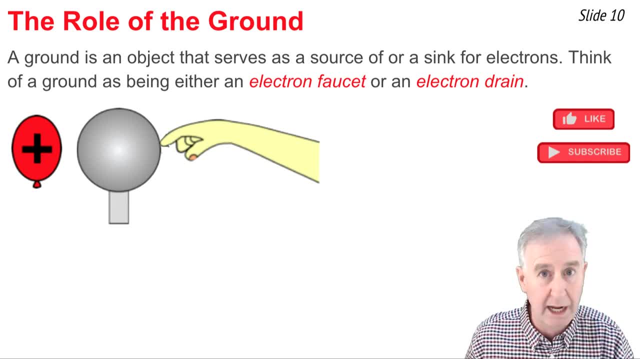 then that's opposites attract, That's a negative electron will be attracted to the positively charged balloon. So that's where the hand acts as the sink or as the source, And electrons flow from the source into the object X, the sphere, And that causes object X to be charged negatively. 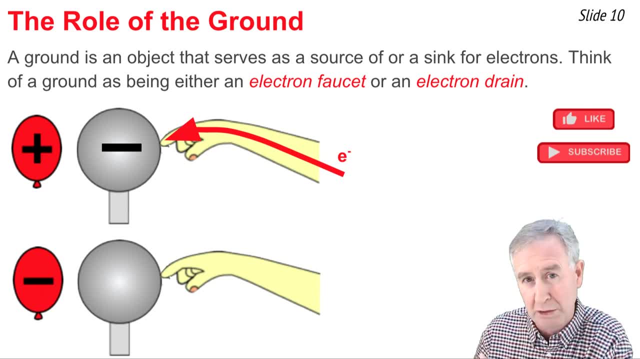 But if you have a negatively charged object held next to the neutral sphere, electrons in the sphere see it and they say: oh, I'm negative, Oh, that's repulsive. But if you have a negatively charged object held out of the sphere into the ground and that causes the sphere, 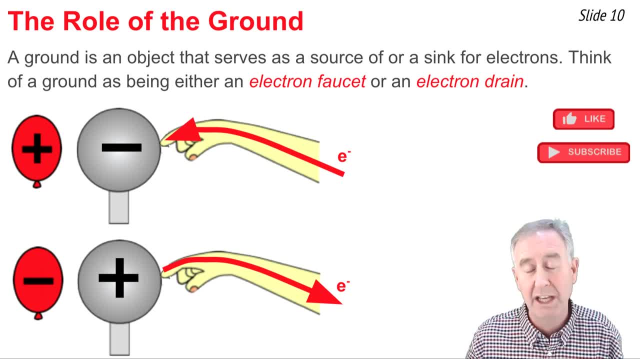 to become charged positively as a result of the loss of its electrons. In this situation, the ground is acting as the sink. Now the best grounds are large enough to contain a lot of electrons and spread them out as far away as possible. That makes one of the best grounds. 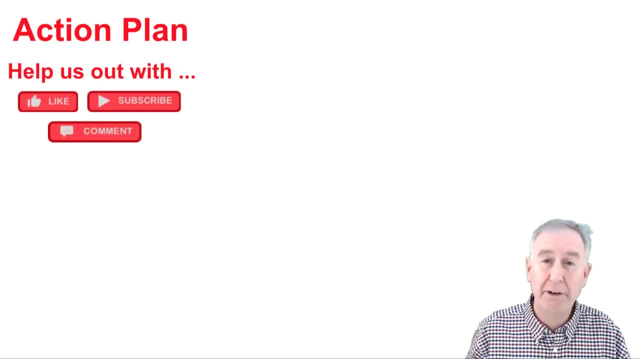 around the ground or the Earth. It's at this time of every video that I try to give you an action plan, a series of next steps making the learning stick. But before I help you out with that, could you help us out by giving us a like or subscribing to the channel? 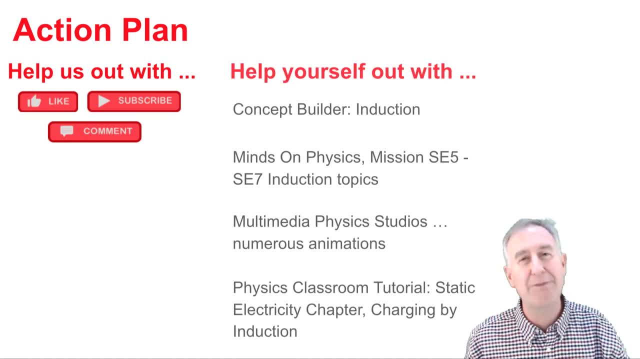 or even leaving a question or comment in the comments section below. Now for your action plan. Here are four items that you can find on our website. Links to each of these items can be found in the description section of this video. Any one of them would be great follow ups to this video. 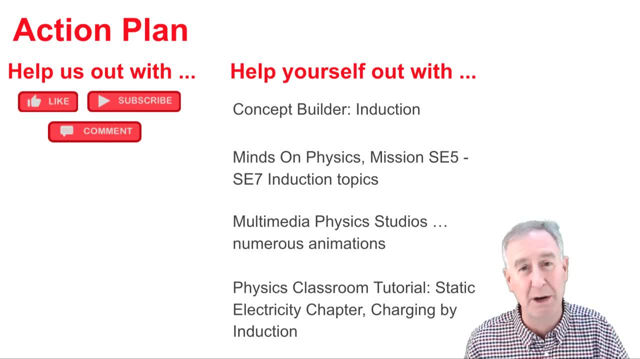 on charging by induction, So pick one that suits your need and give it a try. Whatever you do, I wish you the best of luck. My name's Mr H And thank you for watching.